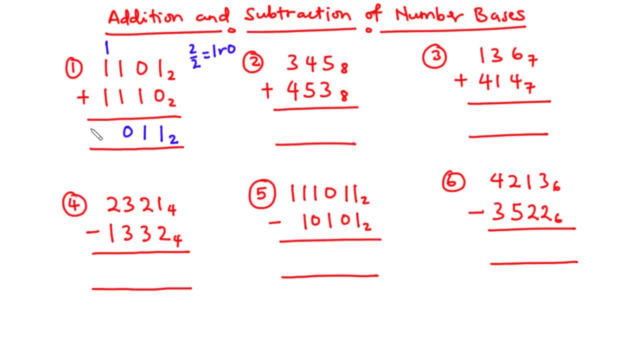 Now, one plus one is two. Two plus one is three. So because three is greater than or equal to two, we are going to divide three by base two And this is equal to one remainder one. So we write the remainder here and then we carry on the one. 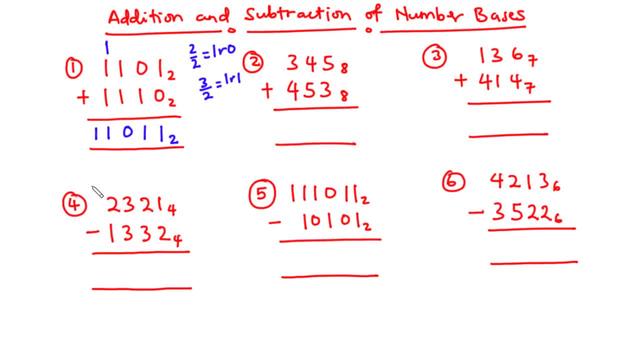 Now one plus zero. zero is still one. So we have our final answer to be one one zero. one one Base two after adding these two values. Now let's solve for the second one. Here we are working in base eight. Five plus three is eight. 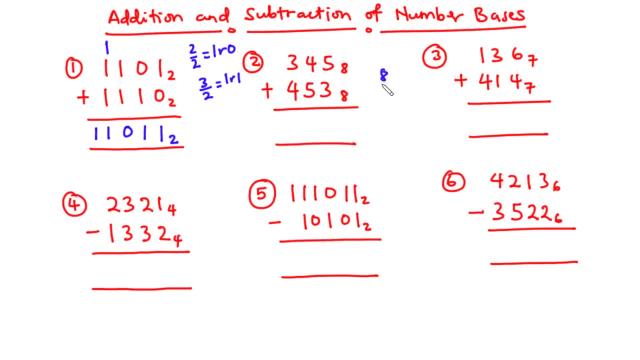 Because we have eight, we can't write eight here. So we divide eight by base eight, and then we have one remainder zero. So we write the remainder here and then we carry on this. one One plus four is five. Five plus five is ten. 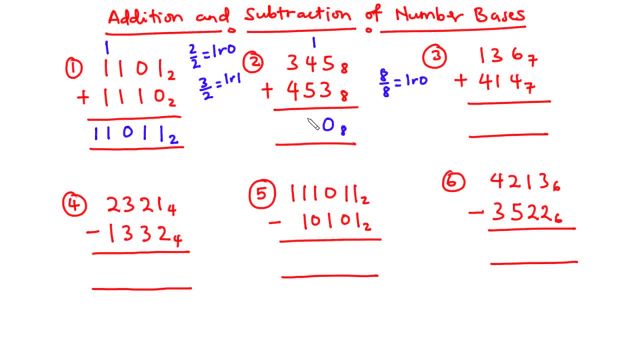 Ten divided by eight is one, remainder two. So we write two, and then we carry on one. One plus three is four. Four plus four is eight, So we write the remainder, which is zero, and then we carry on one. Now, one plus zero, zero is one. 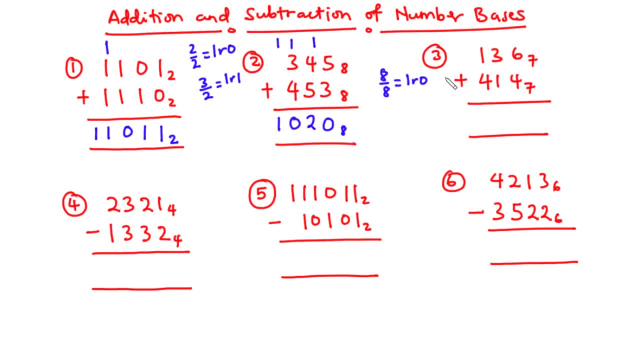 So we have one zero two, zero base eight. Now to the third one. We are working in base seven. Six plus four is ten. Ten plus four is eight. Ten divided by seven is one, remainder three. So we have the remainder here and then we carry on one. 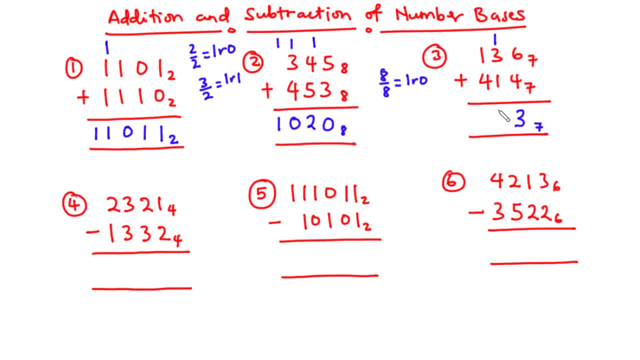 One plus three is four. Four plus one is five. Five is less than seven, so we write the five and then one plus four is also five. Now let's move on to subtraction. So for example, four Here, because we are working in base four, whatever we borrow- is four, not ten. 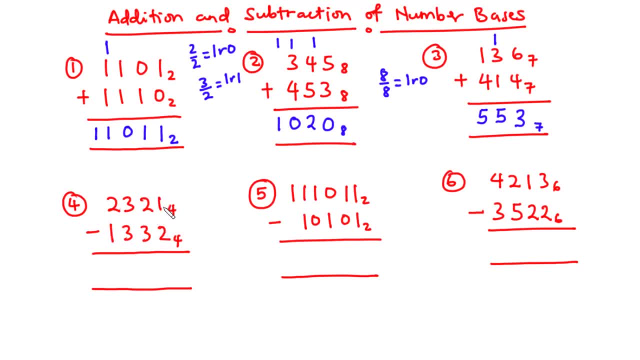 So we have two minus two. It's not possible because one is less than two, So we need to borrow from the next value, which is two. So when we borrow from two, two becomes one, and then what we borrow is four. So we have four plus one, which is five, and then five minus two is three. 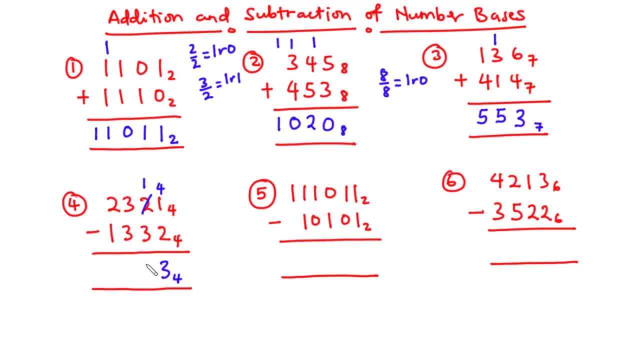 Now we are left with one here. One minus three is not possible because one is less than three. So we borrow from the next value, which is three. Now this becomes 2, and what we borrow is 4.. So 4 plus 1 is 5, 5 minus 3 is 2.. 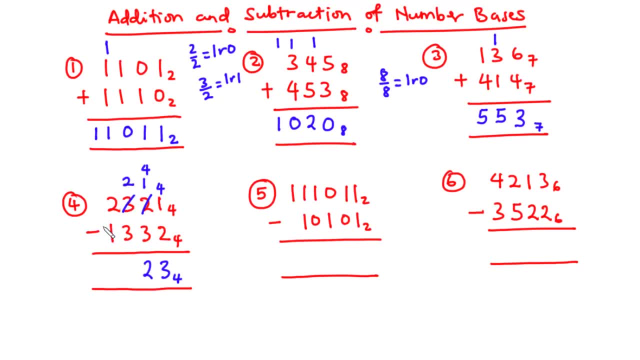 So we have 2 here, Now we have 2.. 2 minus 3 is not possible. we borrow from the next value. This becomes 1, and what we borrow is 4.. So 4 plus 2 is 6,, 6 minus 3 is 3.. 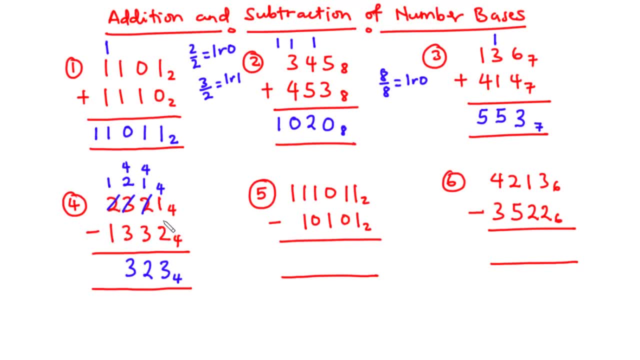 And then here, 1 minus 1 is 0.. So after subtracting 1, 3, 3, 2, base 4 from 2, 3, 2, 1, base 4,, we have our final answer. 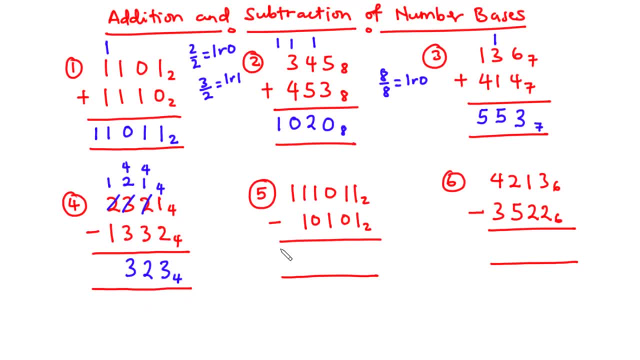 to be 3, 2, 3,, base 4.. Now let's move on to example 5.. We are working in base 2, 1 minus 1 is 0, 1 minus 0 is 1, 0 minus 1, we can't do that. 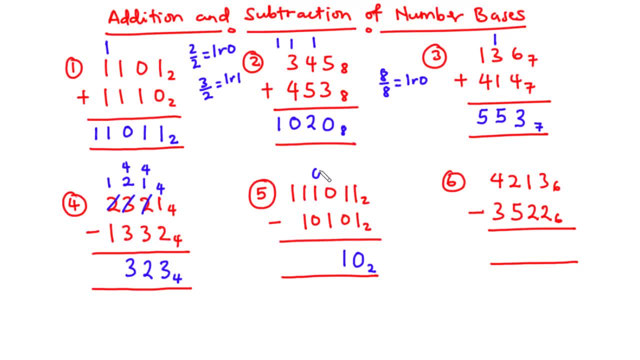 so we need to borrow from the next value, So this becomes 0. And then what we borrow? We need to borrow because we are working in base 2, is 2.. Now 2 minus 1 is 1,, 0 minus 0 is 0,, 1 minus 1 is 0, and then 1 minus 0 is 1.. 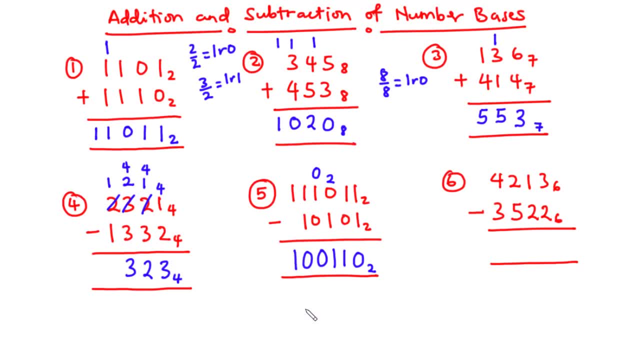 So this is our answer: 1, 0, 0, 1, 1, 0, base 2.. Now to example 6, 3 minus 2 is 1, 1 minus 2 is not possible. we need to borrow from this. 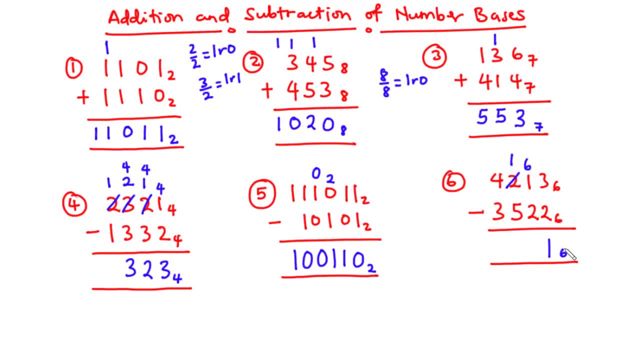 value. So what we borrow is 6, because we are working in base 6.. 6 plus 1 is 7,. 7 minus 2 is 5.. Here we have 1.. So we need to borrow from this value. 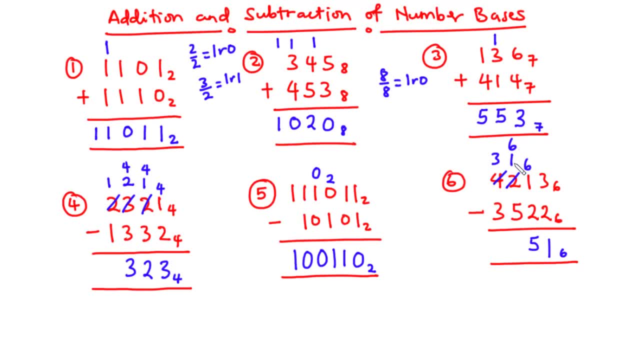 So this becomes 3. And then we borrow 6.. So 6 plus 1 is 7,, 7 minus 5 is 2.. And then 3 minus 3 is 0,. so we have 2, 5, 1 base 6.. 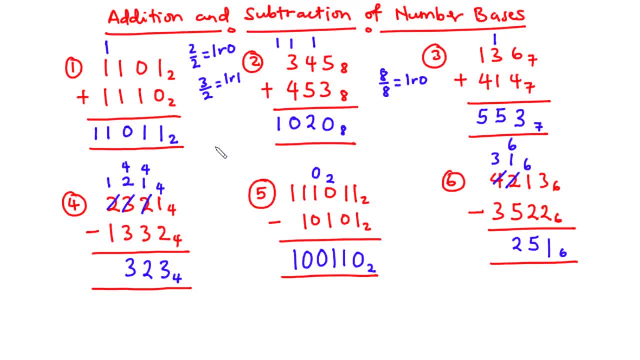 So basically, this is how to perform addition- Thanks for watching- and subtraction of other number bases. Now let's move on to the next section where we are going to solve more complex examples. Now let's solve example 7.. The dimensions of a rectangle are: 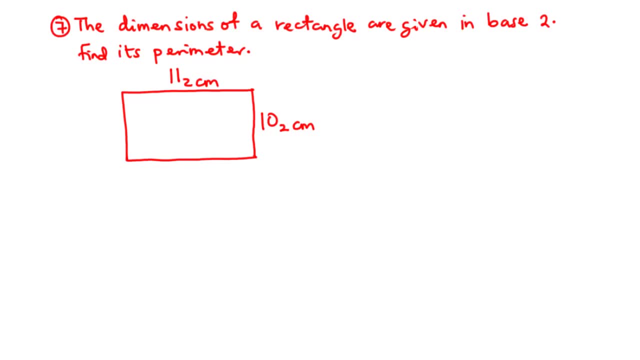 given in base 2.. Find its perimeter. So here we have a rectangle with a length 11 base 2 centimeters and then with a width, 10 base 2 centimeters. Now we are going to find the perimeter of this rectangle in base 2.. Now the perimeter of a rectangle is given by 2L plus 2W, That is 2 times. 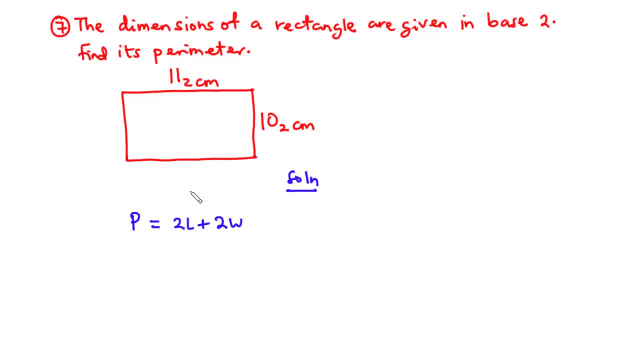 the length plus 2 times the width. Now, because we've not done multiplication of number bases, we can expand this expression so that we have L plus L plus W plus W. So let's substitute these values. So L is the length, That is, 11 base 2 centimeters, and then we have the width, W, to be 10 base 2. 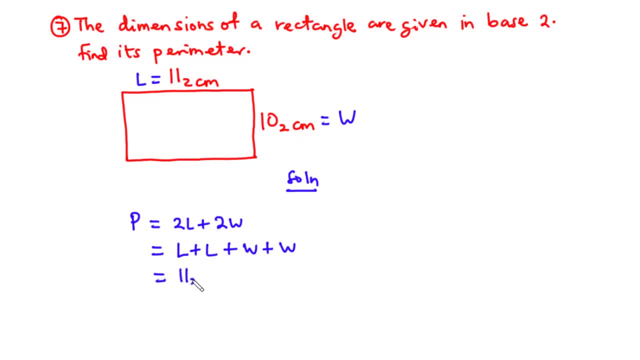 centimeters. So we have 11 base 2 plus 11 base 2 plus 10 base 2 plus 10 base 2.. Now let's work it out here: 11 base 2 plus 11 base 2 plus 10 base 2 plus 10 base 2.. So we have 11 base 2 plus 11 base 2. 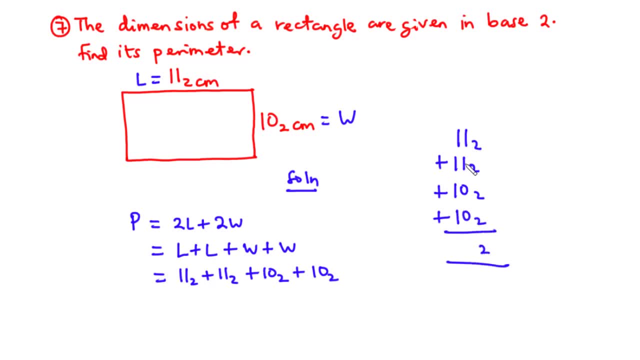 1 plus 1 is 2.. 2 plus 0 is 2, and then 2 plus 0 is also 2.. Now, because we are working in base 2, we are going to divide the value that we have by the base, So that is 1 remainder 0.. So we have the remainder here, and then we carry on. the 1. 1 plus 1 is 2.. 2 plus 1 is 3.. 3 plus 1 is 4.. And then 4 plus 1 is 5.. Now, because 5 is greater than 2, we are going to divide the value that we have by the base, So that is 1 remainder 0.. So we have the remainder here, and then we carry on. the 1. 1 plus 1 is 2.. 2 plus 1 is 3.. 3 plus 1 is 4.. And then 4 plus 1 is 5.. Now, because 5 is greater than 2, we are going to divide the value that we have by the base, So that is 1 remainder 0. So we have the remainder here, and then we carry on. the 1. 1 plus 1 is 2.. 2 plus 1 is 3.. 3 plus 1 is 4.. And then 4 plus